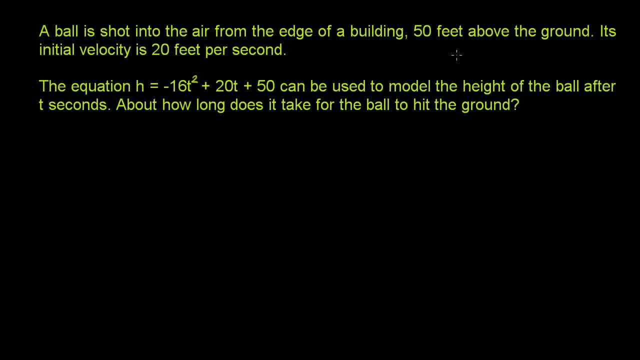 A ball is shot into the air from the edge of a building 50 feet above the ground. Its initial velocity is 20 feet per second. The equation h- and I'm guessing h is for height- is equal to negative. 16t squared plus 20t plus 50 can be used to model the height of the ball. 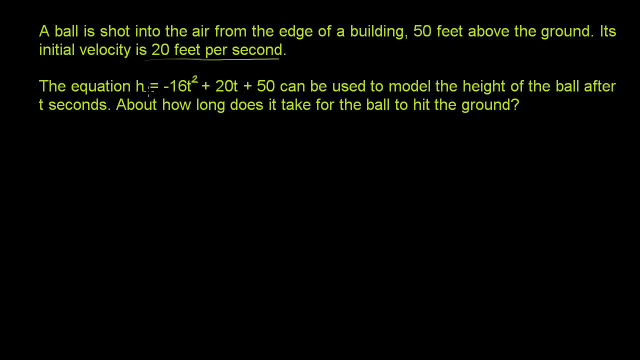 after t seconds. And I think in this problem they just want us to accept this formula, although we do derive formulas like this and show why it works for this type of problem in the Khan Academy Physics playlist. but for here we'll just go with the flow on this example. 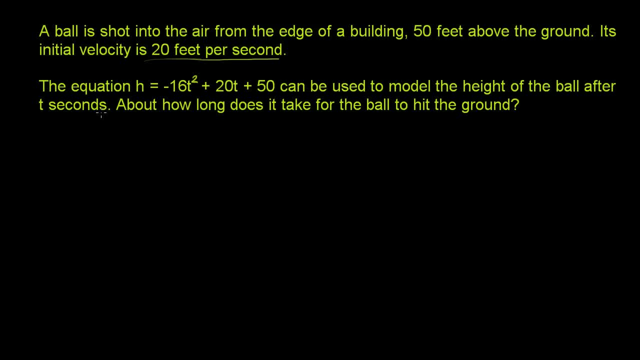 So they give us the equation that can be used to model the height of the ball after t seconds and then say about how long does it take for the ball to hit the ground? So if this is the height, the ground is when the height is equal to zero. So hitting the ground means this, literally means 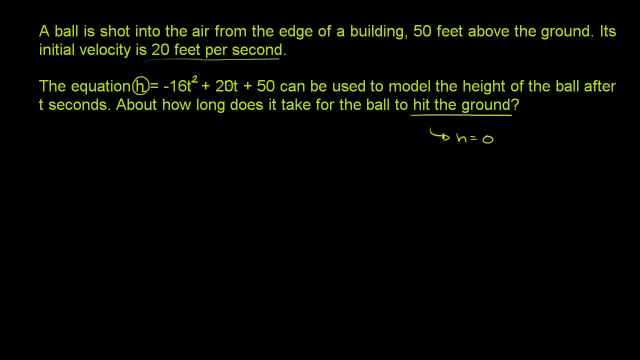 that h is equal to zero. So we need to figure out what times, at which times, does h equal zero? So we're really solving the equation: zero is equal to negative, 16t squared plus 20t plus 50.. And if you want to simplify this a little bit, let's see: everything here is divisible, at least. 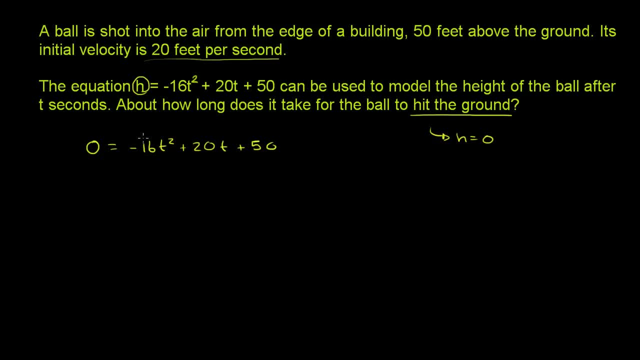 by two And let's divide everything by negative two, just so that we can get rid of this negative leading coefficient. So you divide the left-hand side by negative two, you still get a zero Negative. 16 divided by negative two is eight. So eight t squared 20 divided by negative two. 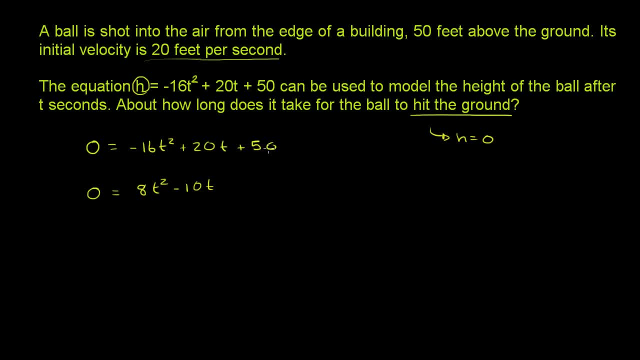 is negative 10, minus 10t. 50 divided by negative two is minus 25.. And so we have eight t squared minus 10t. minus 25 is equal to zero, If you're comfortable with this on the left-hand side. 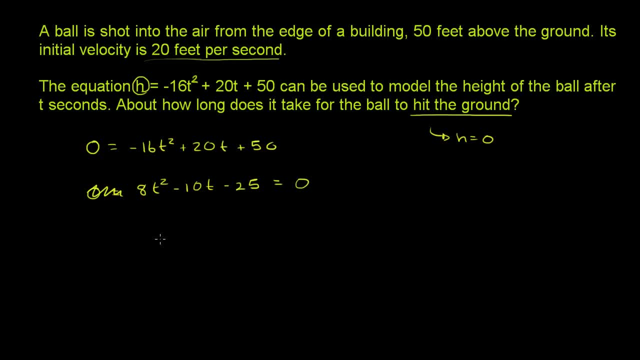 we can put it on the left-hand side. We could just say: this is equal to zero And now we solve And we could complete the square here. or we can just apply the quadratic formula which is derived from completing the square, And we have this in standard form. We know that this is our a. 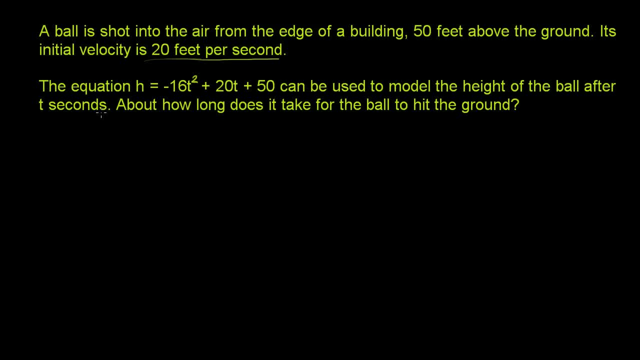 So they give us the equation that can be used to model the height of the ball after t seconds and then say about how long does it take for the ball to hit the ground? So if this is the height, the ground is when the height is equal to zero. So hitting the ground means this, literally means 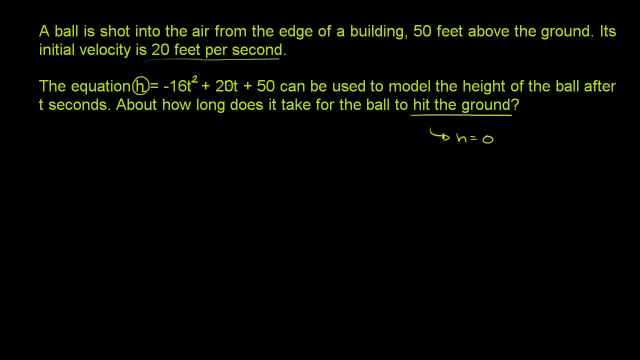 that h is equal to zero. So we need to figure out what times, at which times, does h equal zero? So we're really solving the equation: zero is equal to negative, 16t squared plus 20t plus 50.. And if you want to simplify this a little bit, let's see: everything here is divisible, at least. 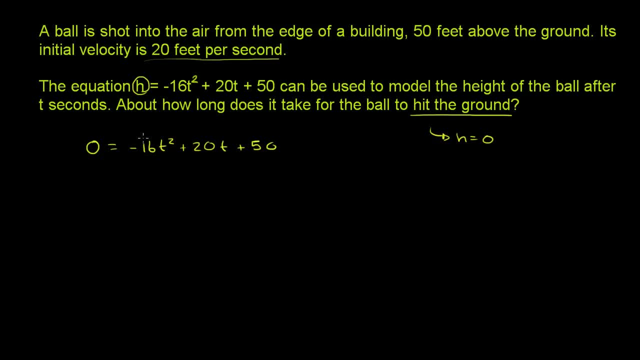 by two And let's divide everything by negative two, just so that we can get rid of this negative leading coefficient. So you divide the left-hand side by negative two, you still get a zero Negative. 16 divided by negative two is eight. So eight t squared 20 divided by negative two. 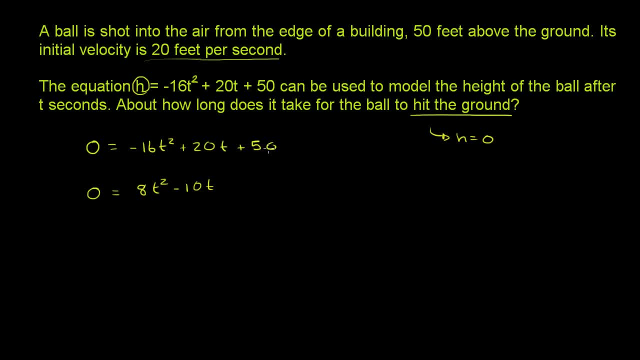 is negative 10, minus 10t. 50 divided by negative two is minus 25.. And so we have eight t squared minus 10t. minus 25 is equal to zero, If you're comfortable with this on the left-hand side. 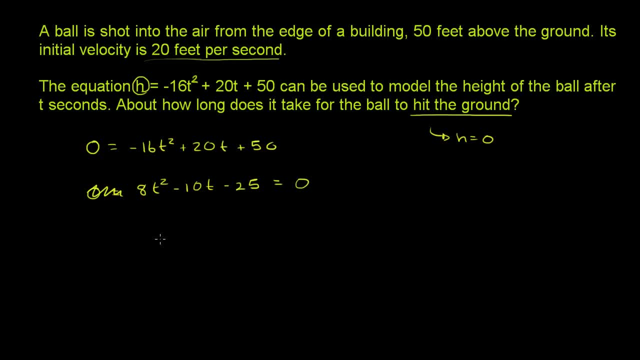 we can put it on the left-hand side. We could just say: this is equal to zero And now we solve And we could complete the square here. or we can just apply the quadratic formula which is derived from completing the square, And we have this in standard form. We know that this is our a. 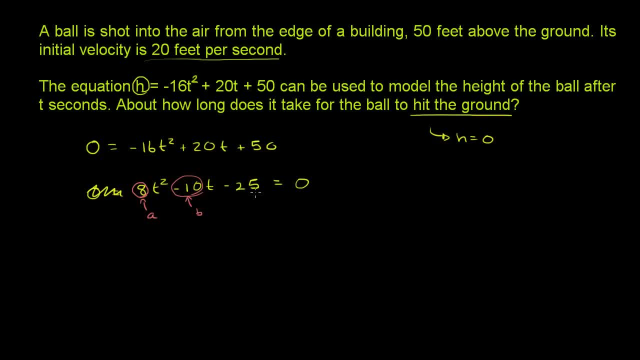 this right over here is our b and this over here is our c, And the quadratic formula tells us that the roots- and in this case it's in terms of the variable t- are going to be equal to negative b plus or minus the square root of b squared minus 4ac. all of that over 2a. So if we apply it, 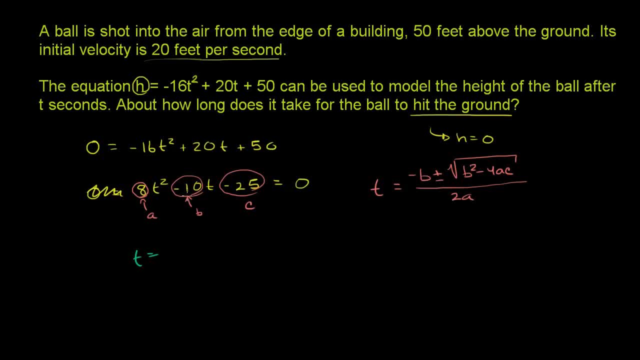 we get: t is equal to negative b, b is negative 10, so negative, negative 10.. So negative, negative 10 is going to be positive 10 plus or minus the square root of negative 10. squared well, that's just positive 100, minus 4 times a, which is 8, times c, which is negative 25.. 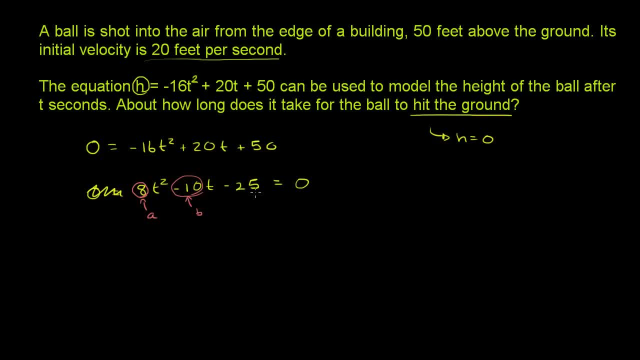 this right over here is our b and this over here is our c, And the quadratic formula tells us that the roots- and in this case it's in terms of the variable t- are going to be equal to negative b plus or minus the square root of b squared minus 4ac. all of that over 2a. So if we apply it, 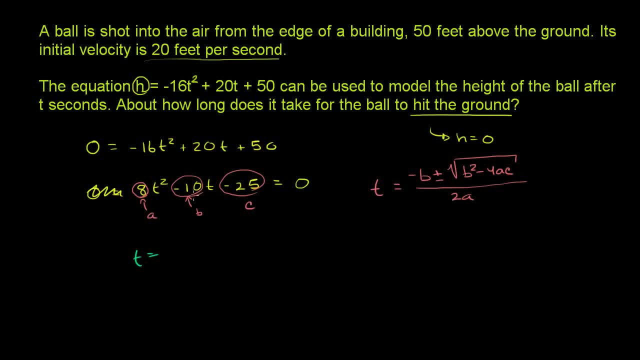 we get: t is equal to negative b, b is negative 10, so negative, negative 10.. So negative 10 is going to be positive 10 plus or minus the square root of negative 10. squared well, that's just positive 100, minus 4 times a, which is 8, times c, which is negative 25.. 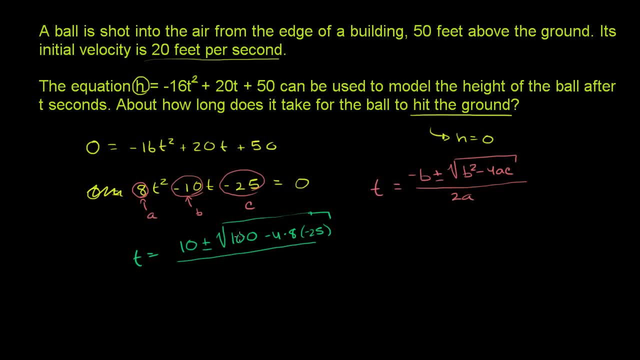 Negative: 25.. And all of that over 2a a is 8, so 2 times 8 is 16.. And this over here we have a. let's see if we can simplify this a little bit. The negative sign: negative times: a negative. 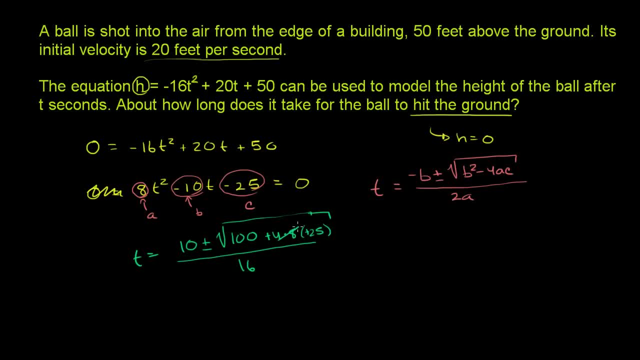 these are going to be positive ��는, So negative minus 9 times 25 is 100, times 8 is 800, so all of that simplifies to 800, and we have 100 plus 800 under the radical sign. So this is equal to 10 plus or minus the. 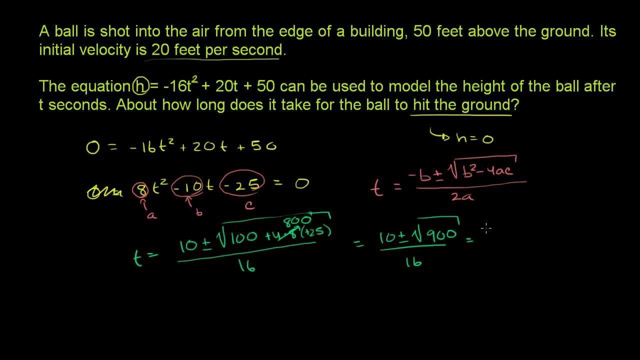 square root of 900, all of that over 16. And this is equal to 10 plus or minus. square of 900 is 30 over 16.. And so we get: time is equal to 10 plus 30 over 16, is 40 over 16,. 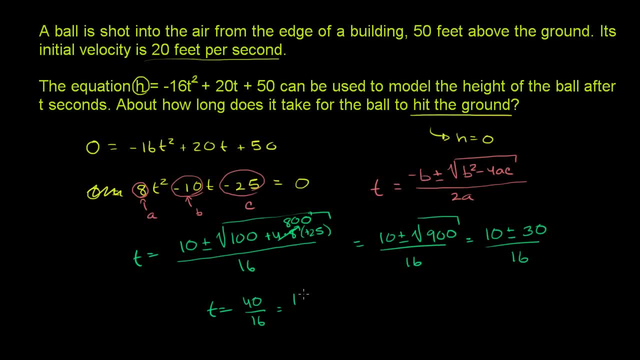 which is the same thing. y. if we divide the numerator and the denominator by 9,, which is 40 over 16,, we can get this too, y by 4 to simplify it as 10 over, or actually, even better, divide it by 8.. 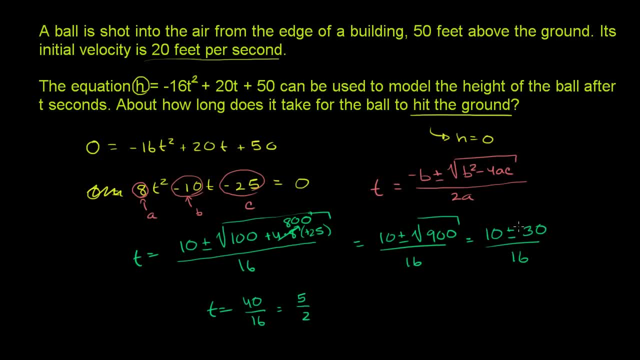 That's 5 over 2.. So that's one solution. If we add the 30,, if we subtract the 30, we'd get 10 minus 30. Or t is equal to 10 minus 30,, which is negative: 20 over 16.. 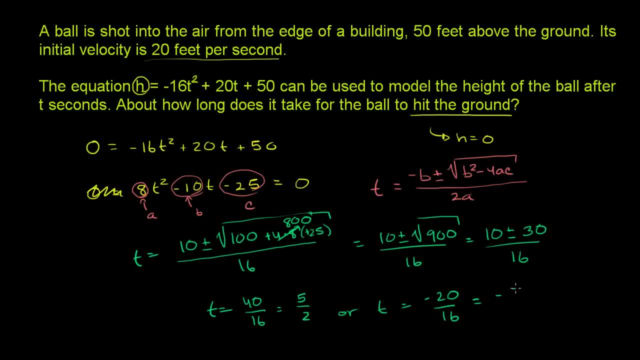 Divide the numerator and the denominator by 4, you get negative 5 over 4.. Now we've got to remember, we're trying to find a time, And so a time at least in this problem that we're dealing with, we should only 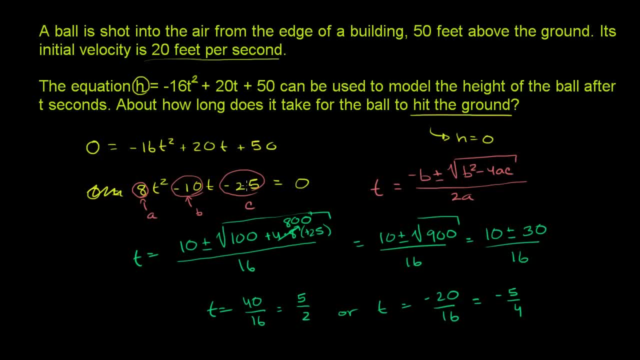 think about positive times. We want to figure out how much time has taken Pat, how long does it take for the ball to hit the ground? We don't want to go back in time, So we don't want our negative answer right here. 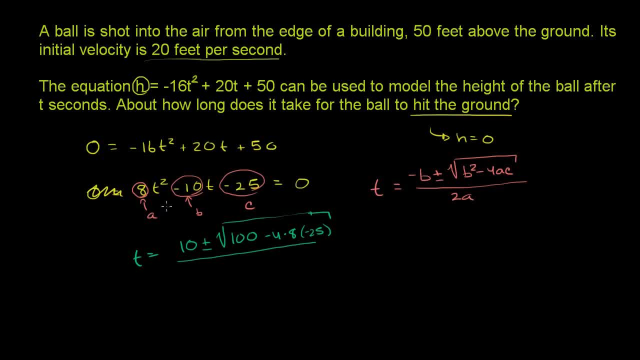 Negative 25.. And all of that over 2a a is 8.. So 2 times 8 is 16.. And this over here we have a- let's see if we can simplify this a little bit. The negative sign: negative times a negative. 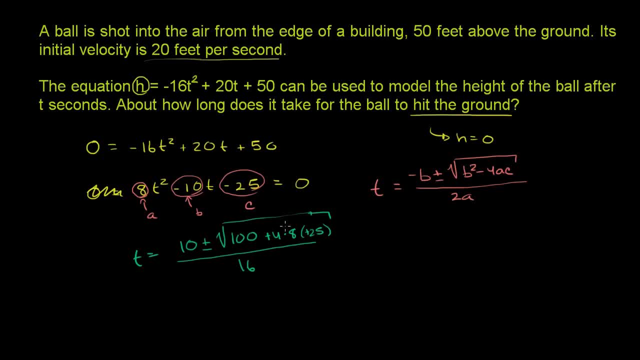 these are going to be positive 4 times a negative. these are going to be positive 4 times a negative. these are going to be positive 4 times 25 is 100, times 8 is 800. So all of that simplifies to 800. And we have 100 plus 800 under. 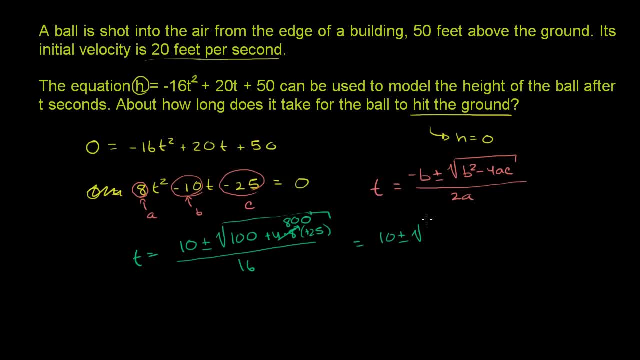 the radical signs. So this is equal to 10 plus or minus the square root of 900, all of that over 16. And this is equal to 10 plus or minus. square root of 900 is 30 over 16.. And so we get: time is equal. 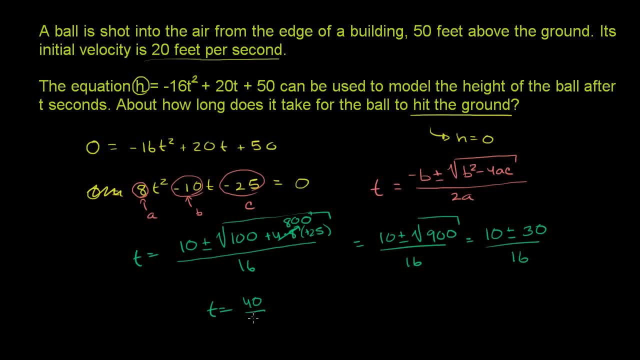 to 10 plus 30 over 16 is 40 over 16, which is the same thing. if we divide the numerator and denominator by 4, to simplify it as 10 over, or actually even better, divide it by 8.. That's 5 over 2.. 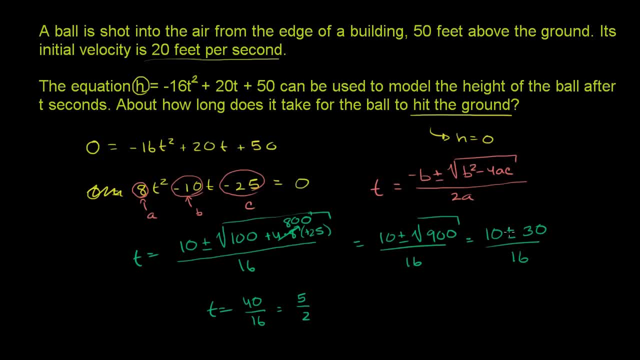 So that's one solution. If we add the 30,, if we subtract the 30, we'd get 10 minus 30. So or t is equal to 10 minus 30, which is negative 20 over 16.. Divide the numerator. 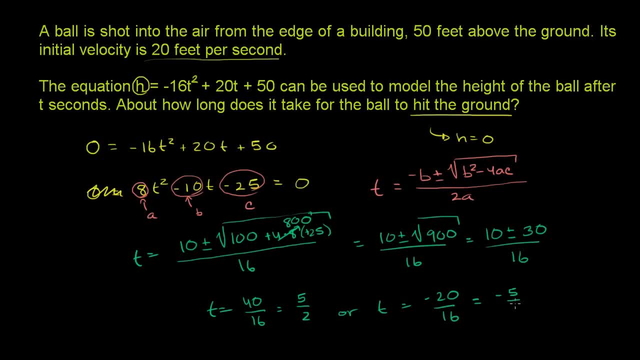 and the denominator by 4, you get negative 5 over 4.. Now we have to remember this was we're trying to find a time, And so a time at least, in what? in this problem, this problem that we're dealing with, we should only think about positive times. We want to figure. 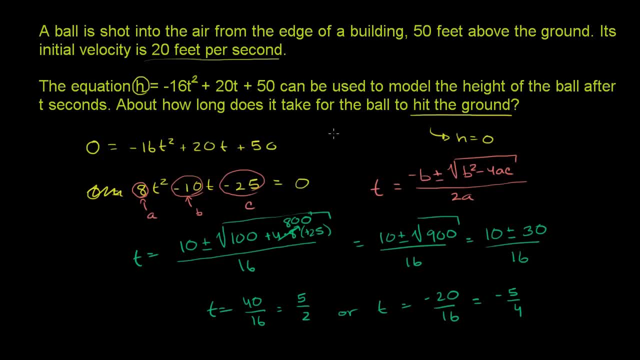 out how much time has taken, Pat, how long does it take for the ball to hit the ground? We don't want to go back in time, So we don't want our negative answer right here, So we only want to think about our positive answer. And so this tells us that the only route that should work is 5 halves. 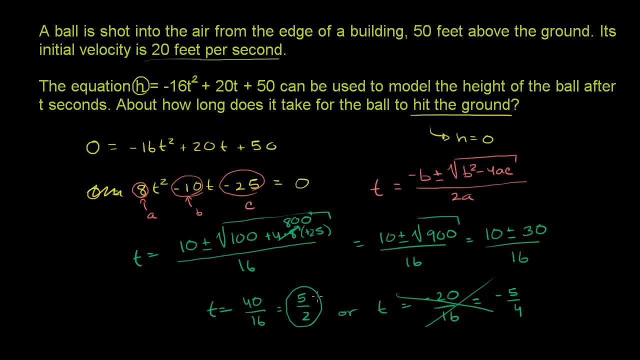 And we assume that this is in seconds, So this is in 5 halves seconds. I wouldn't worry too much about the physics here. I think they really just want us to apply the quadratic formula to this modeling situation. The physics: we go into a lot more depth and give you the kind of 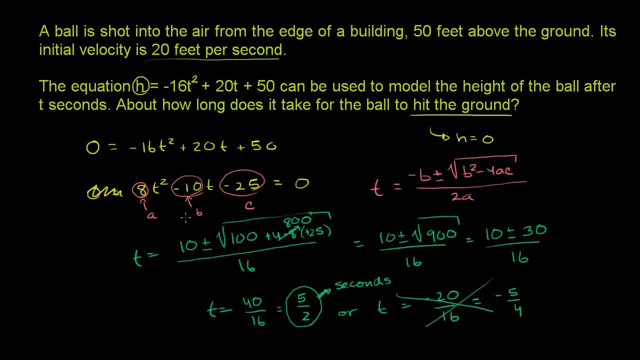 the conceptual understanding on the on our physics playlist. But let's verify that we definitely are at a height of zero at 5 halves seconds. Or if t is equal to 5 halves, this expression right over here does give us h is equal to zero. So we have, let's try it out, We have. 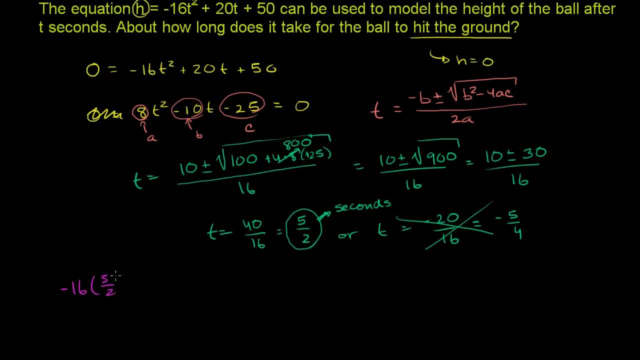 negative: 16 times 5 halves squared. times 5 halves squared plus 20 times 5 halves plus 50.. This is going to be equal to this needs to be equal to. This is going to be equal to. this needs to be. 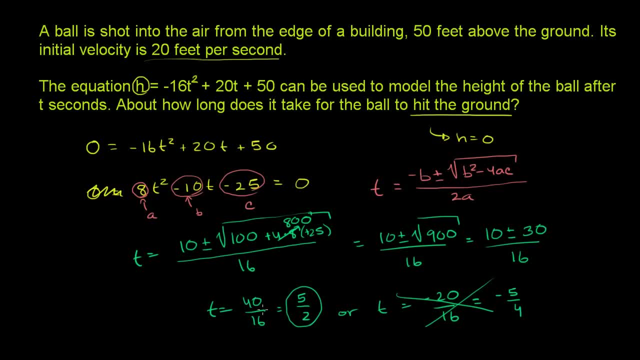 So we only want to think about our positive answer, And so this tells us that the only route that should work is 5 halves, and we assume that this is in seconds, So this is in 5 halves seconds. I wouldn't worry too much about the physics here. 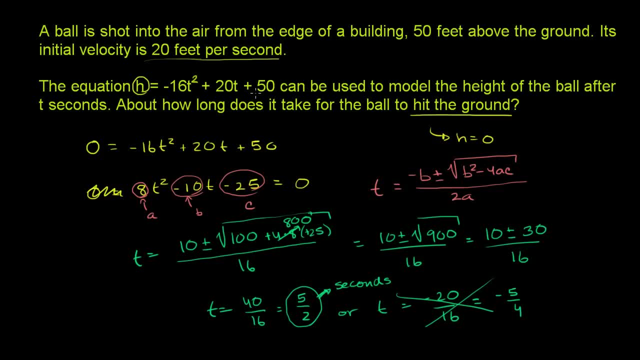 I think they really just want us to apply the quadratic formula to this modeling situation. The physics: we go into a lot more depth and give you the conceptual idea. You'll get a full understanding on our physics playlist, But let's verify that we definitely 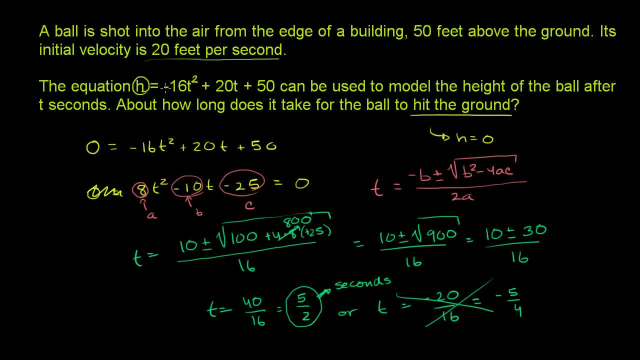 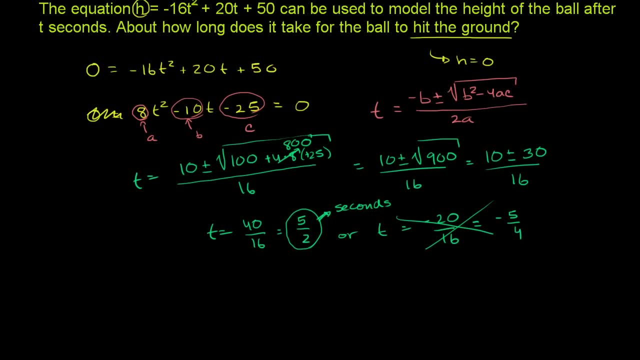 are at a height of 0 at 5 halves seconds. Or if t is equal to 5 halves, this expression right over here does give us h is equal to 0.. So we have- let's try it out- We have negative 16 times 5 halves squared. 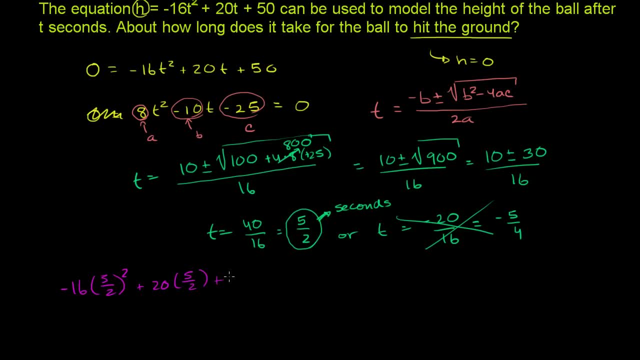 plus 20 times 5, halves plus 50. This is going to be equal to. this needs to be equal to 0.. This needs to be equal to 0.. So this is negative 16 times 25 over 4, plus. let's see: 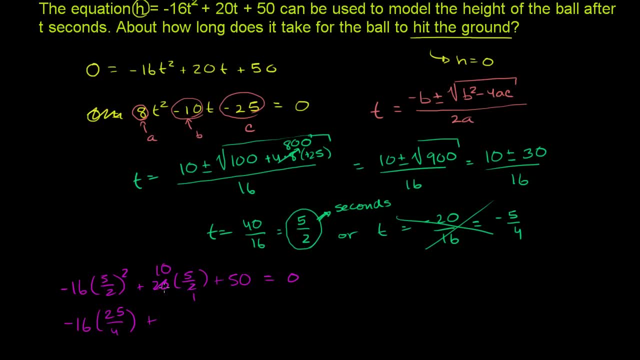 if we divide 20 by 2, we get 10.. If we divide 2 by 2, we get 1.. So 10 times 5 is going to be 50, plus 50. This needs to be equal to 0.. 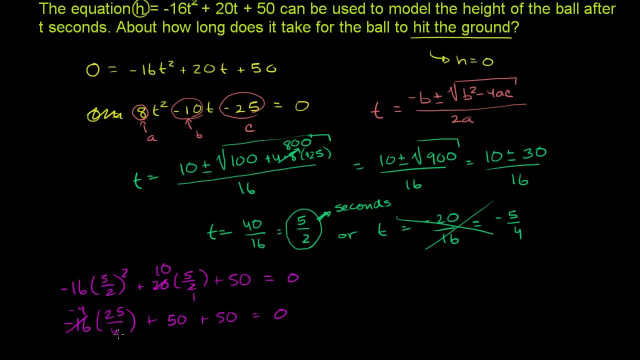 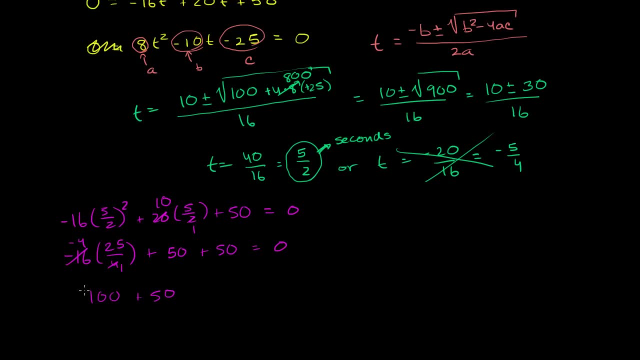 Negative: 16 divided by 4 is negative 4.. 4 divided by 4 is 1.. So you have negative 4 times 25, which is 100, plus 50.. Oh sorry, Negative 4 times 25 is negative 100..